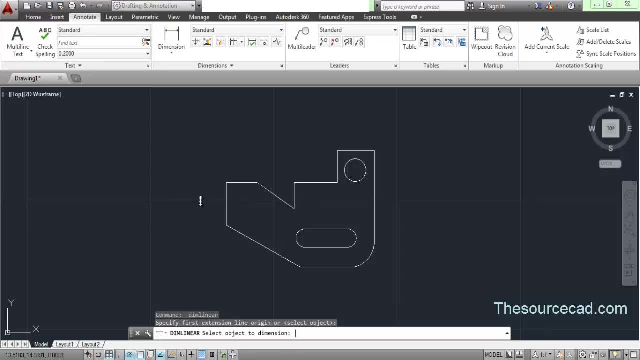 As soon as you press enter, you will see that the cursor changes to the pick box and now you can directly click on the line or arc or circle and the dimension will be mentioned like this. So here we have the dimension directly mentioned. Now let's apply this method again. So I will go to linear and this time press enter and 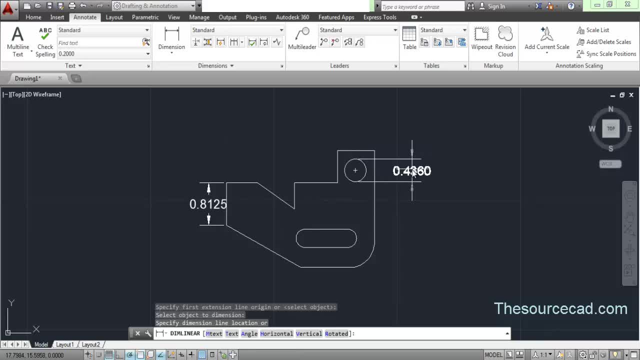 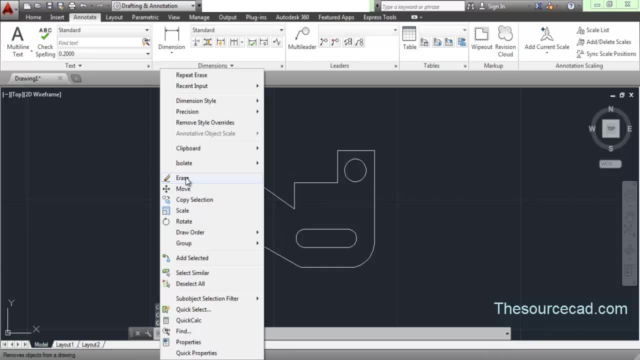 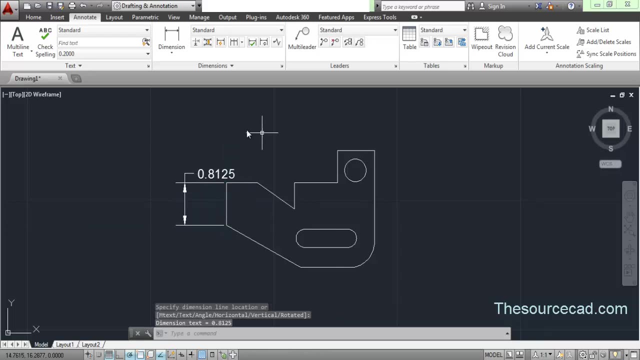 now click on this circle and you will see that the linear dimension of the circle is applied directly. Now we will select points to measure these dimensions. So now go to linear and this time I will select point this point, then this point and drag it, and 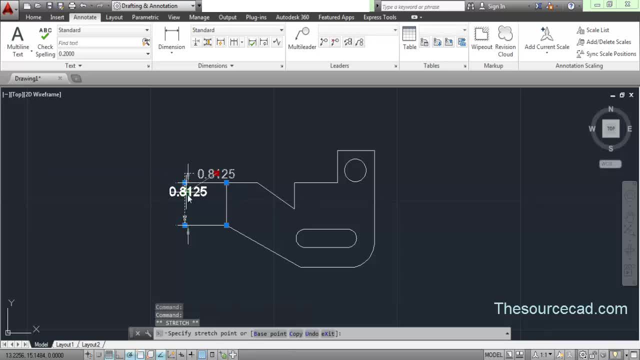 I will apply the dimension. So now, here we have the dimension. So you can apply these dimension using any of the methods which I showed you right now and while using all the other remaining dimension tools. you can apply both of the methods. So now let's go to our next option that was aligned. 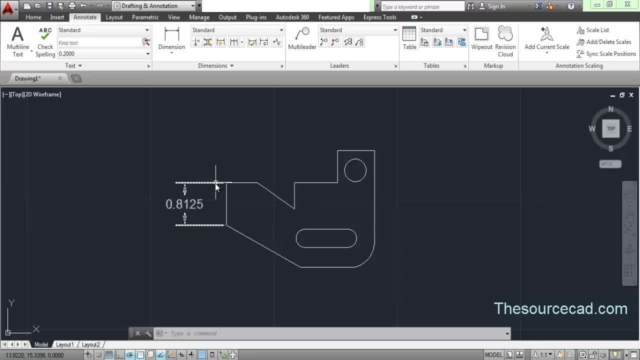 Okay, so we have applied linear dimension, and the linear dimension can be applied only in the case where the object is either vertical or the object is horizontal, like here. in this case, it's horizontal, So the linear dimension can be applied. Now let's first apply linear dimension to this. 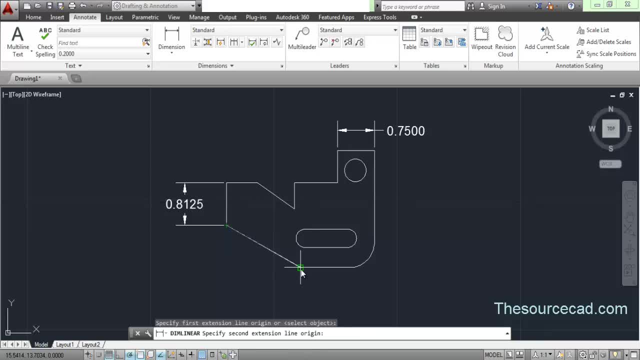 aligned line. Now click on this point, then click on this point, and now you can see that it's making a horizontal dimension. Now let's move on to this direction and it will make a vertical one, but it will not make a dimension which is parallel to this line, So a linear. 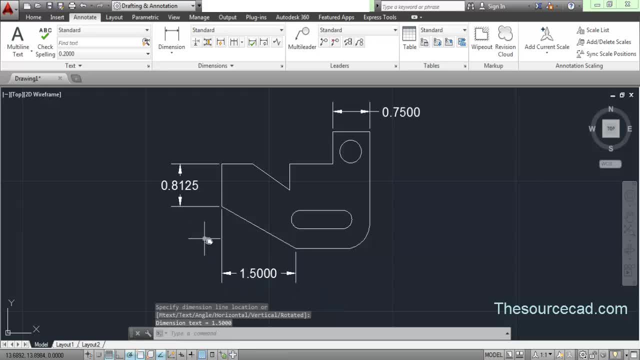 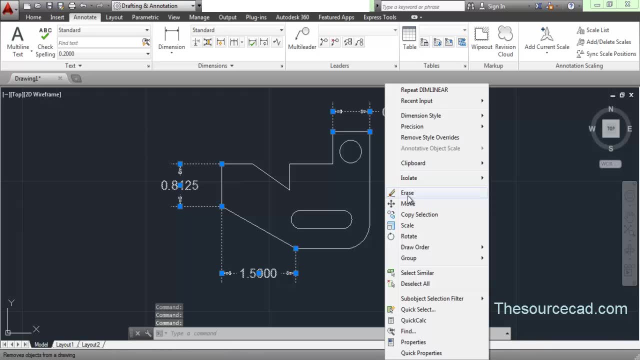 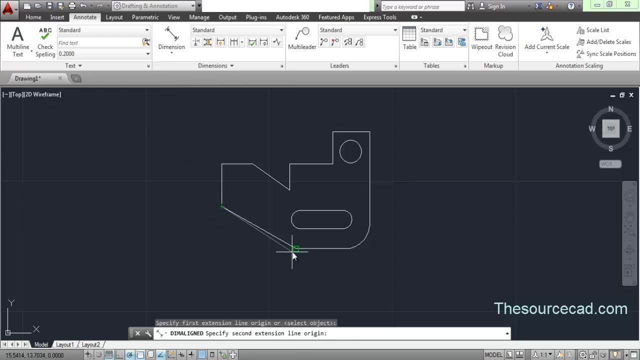 dimension will always make a horizontal or a vertical dimension based upon your direction of cursor, And delete all these dimensions. and now I'll go to aligned. Now click on aligned, and now click on this point and this point. and now, here we have the parallel dimension, which 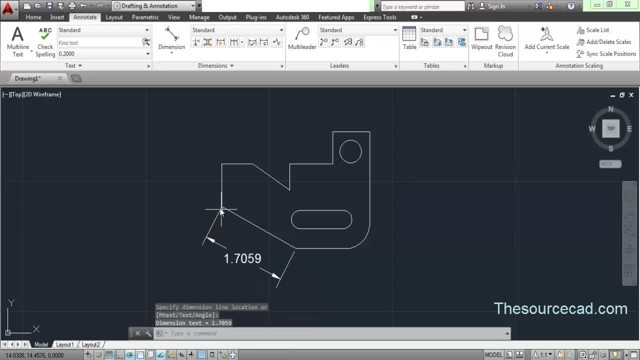 we were looking at. So now you can make a parallel dimension aligned to an angle using this aligned dimension tool. You can make a linear dimension also with this. A linear dimension can also be made using aligned dimension tool. Okay, now let's go and have a look at other dimension commands. So now the next one is: 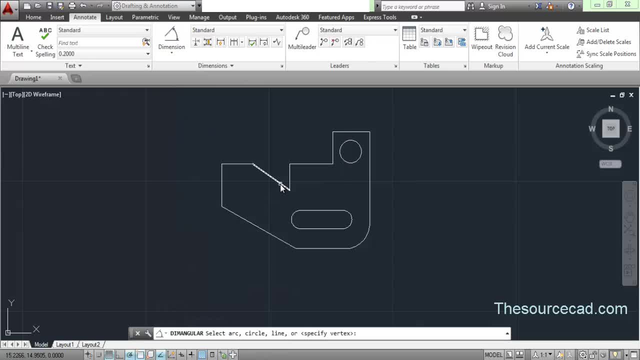 angular. Click on angular and click on first line, then on second line, and here we have the angle between these two lines. The place where you'll click your cursor will signify that angle. So now, if I click on this side, it will be this angle, this angle and this. 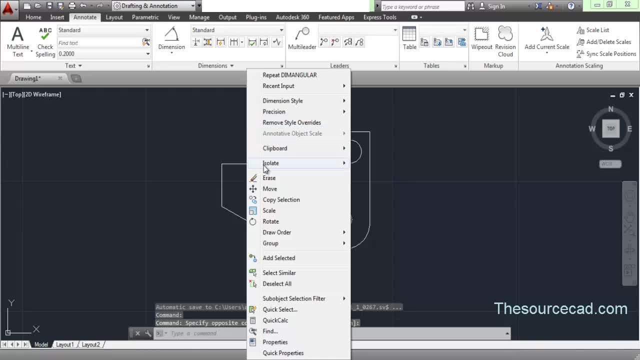 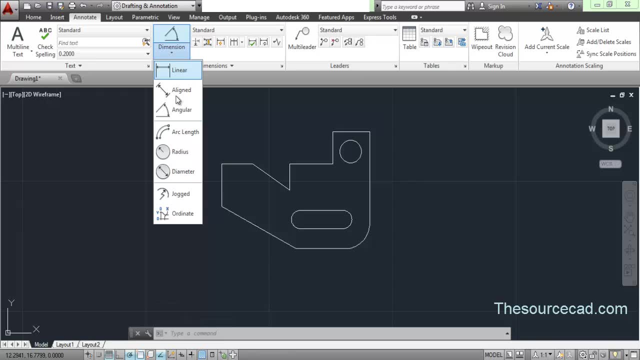 angle. Here I click and here is the angle. In a similar way, you can apply angle to any of the two lines, but make sure those are either lines or polylines, because the angular command will not work if you are using a construction line. So angular command only works for a line. 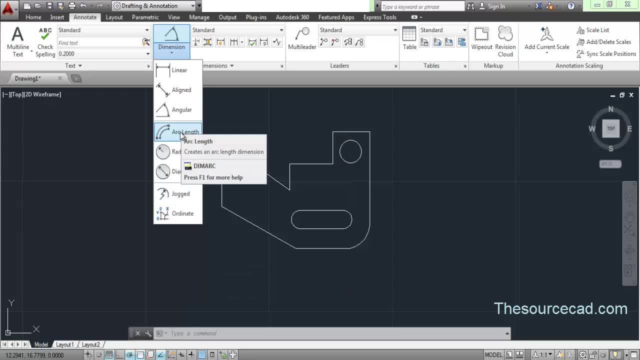 and a polyline. Now let's go to arc length. Now here we have three arcs: The first arc, second arc and the third arc, And using this arc length you can specify length of an arc. So this fillet is an arc. Click on this and there you go, You can see arc length. 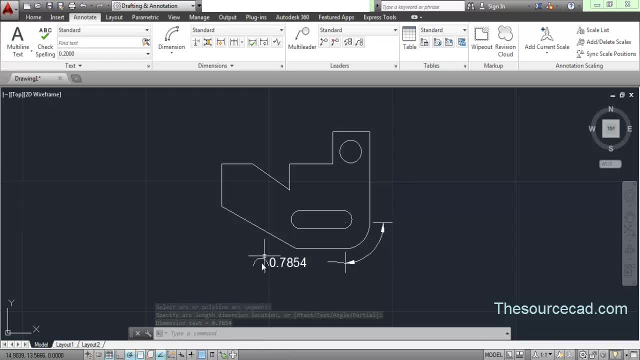 Which is preceded by this arc symbol. Now, the length of this arc is 0.7854.. Make a note that this is a length of arc. This is not the radius or the diameter. We will specify radius and diameter using another command, but this is actually the length of this arc. 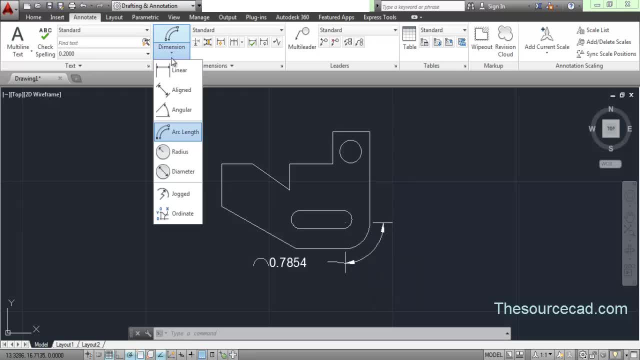 from this point to this point. So now let's go and look at radius. Now click on radius, Click on this arc again, and now you can see that here we have the radius. So the radius of this arc is 0.7854.. 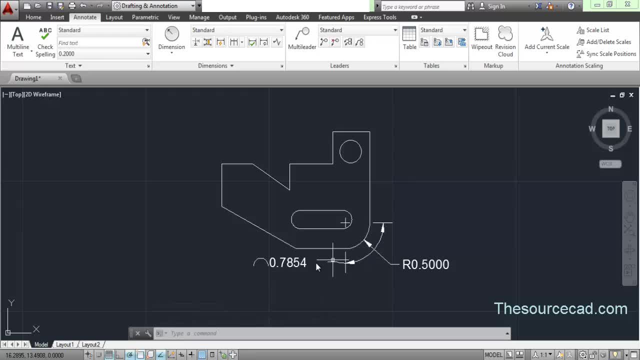 0.5 units and the length of this arc is 0.7854 units and the radius is preceded with r, which signifies that this is a radius. Now let's go to the diameter. click on this arc again, and now you can see that the dimension is preceded with a phi sign, and this indicates it's a diameter and it's 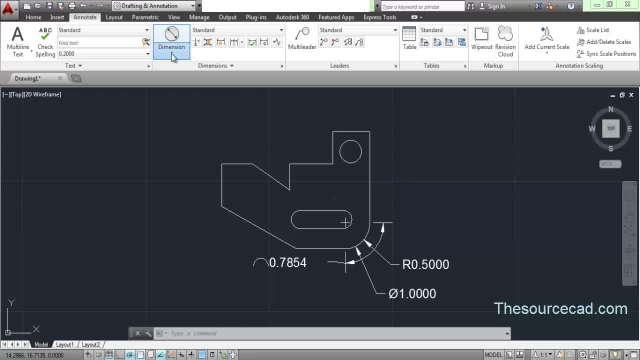 obviously double to radius. You can use these two tools on any of the objects which we have here, like this circle, or you can use it on this arc as well. So now let's go and erase all of these. we don't need it now, Okay. so you have seen all these commands and I will look at these two. 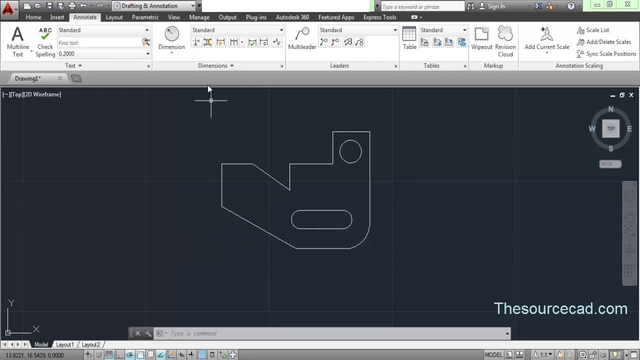 options jogged and ordinate in our next tutorial. and now let's go and have a look at continue and baseline dimensions. For continue dimension, I'll first make a default dimension and then I'll make a default dimension, and then I'll make a default dimension and then